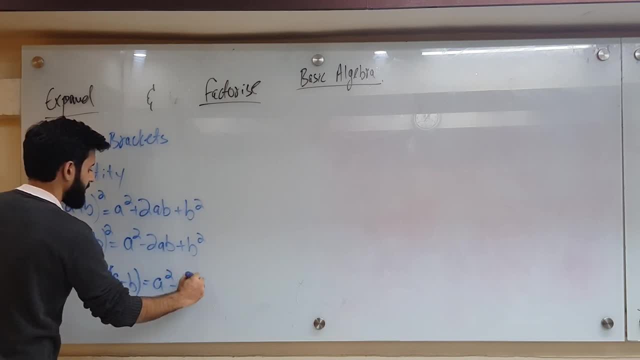 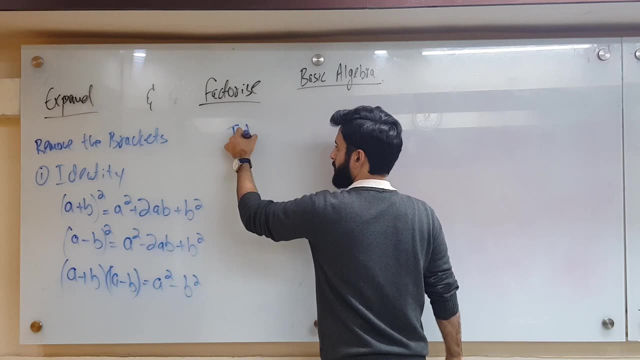 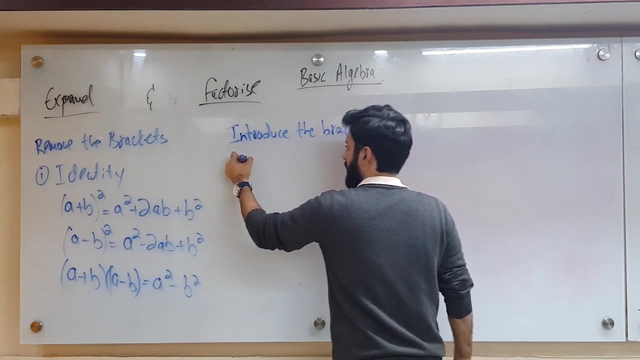 Don't worry, we're going to do plenty of example questions: a squared minus b squared. And then what about? factorize In, factorize- what do we do? We introduce the brackets Again. we can do this with the help of middle term breaking. 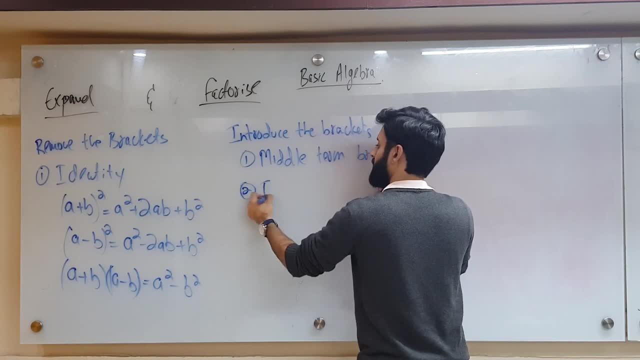 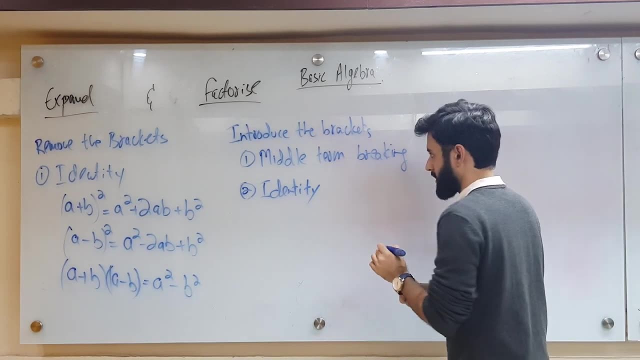 So we can do this with the help of middle term breaking. we can do this with the help of, again, identity. No, no, no, we never factorize with the help of a quadratic formula. We solve with the help of a quadratic formula, but not factorize. 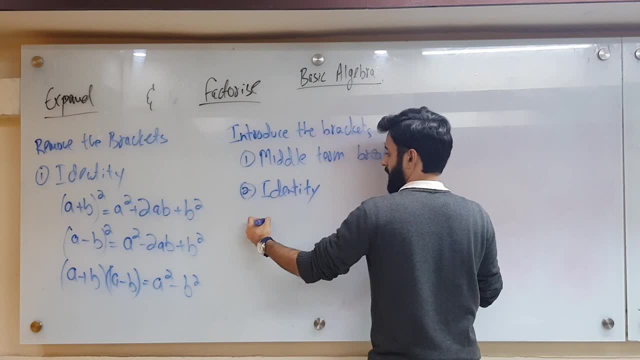 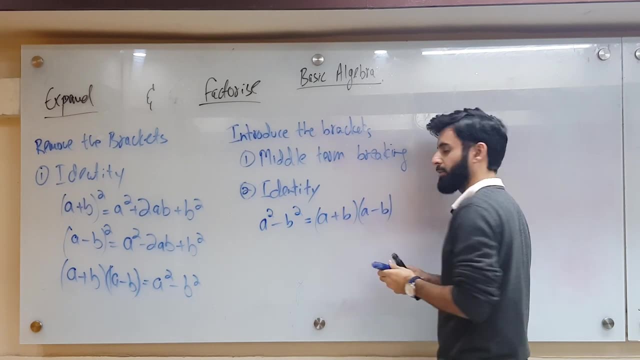 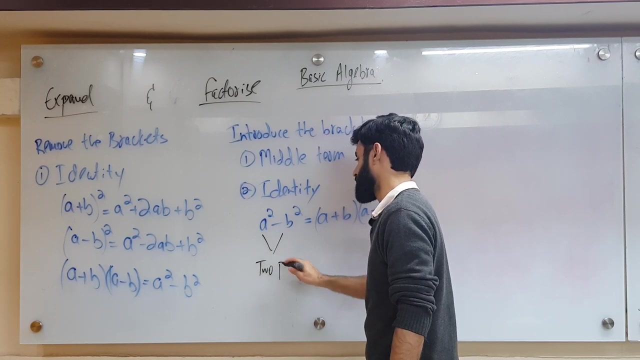 Identity. which identity? This one? your a squared minus b squared equals a plus b, a minus b. So when do we apply this identity? We only apply this identity when you have what's a squared and b squared. These are two perfect squares. 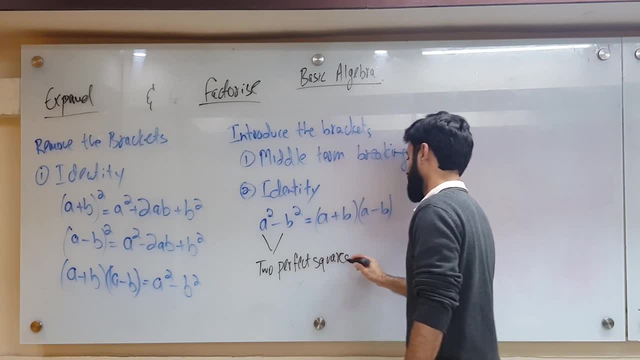 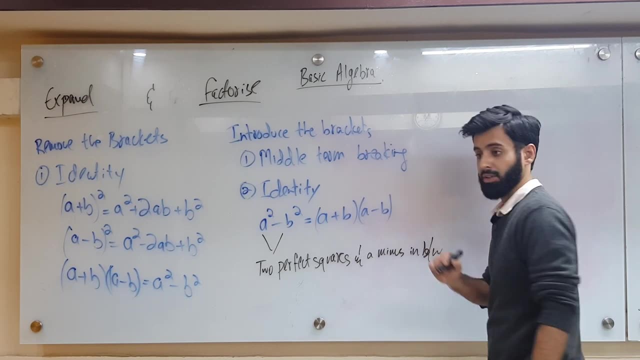 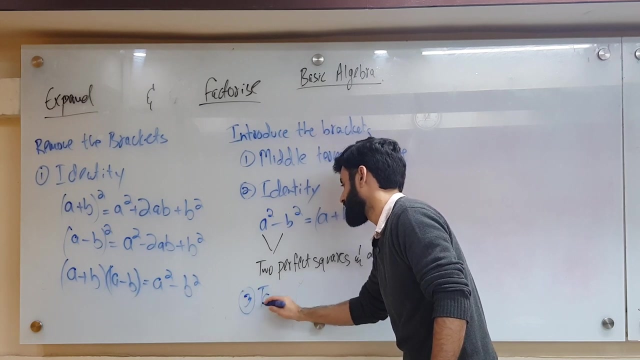 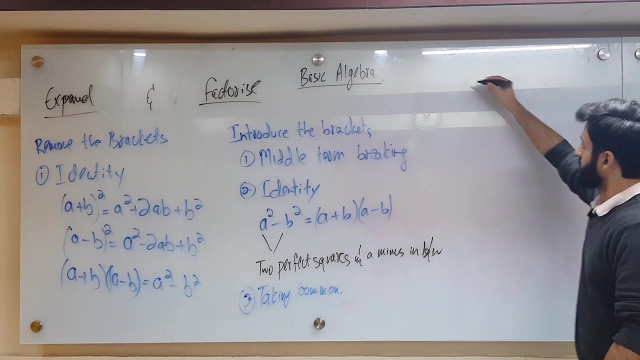 Two perfect squares and a minus in between. You can write these together so that we save time. Yes, yes, keep on writing this. Or you can factorize with the help of taking common, For example. here's example 1.. 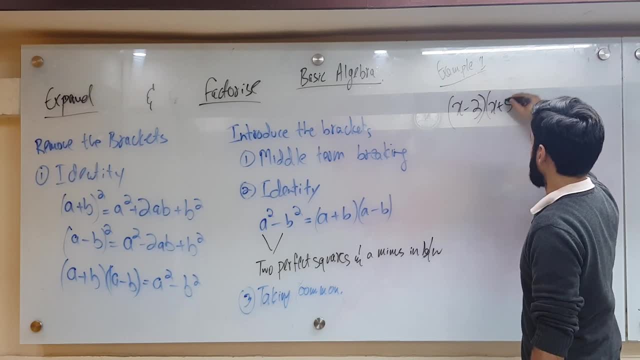 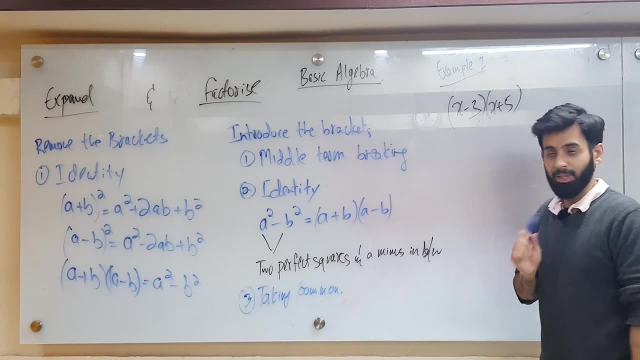 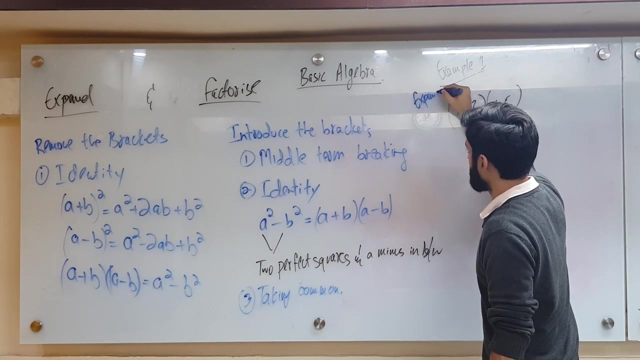 x minus 3, x plus 5.. What will you do with this? Will you factorize it or expand it? No, we will expand it. No, we will expand it because we have to remove the bracket. So a question like this will ask you to do what. It will ask you to expand. 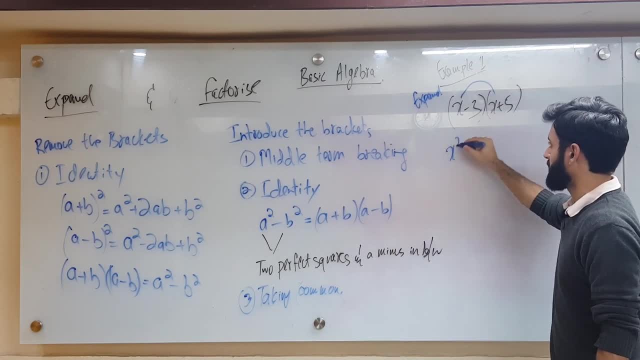 Okay, how can we expand this? This x will get multiplied with this x, So this will give us x squared, and the same x will get multiplied with 5.. So that will give us 5x and then minus 3x, minus 15.. 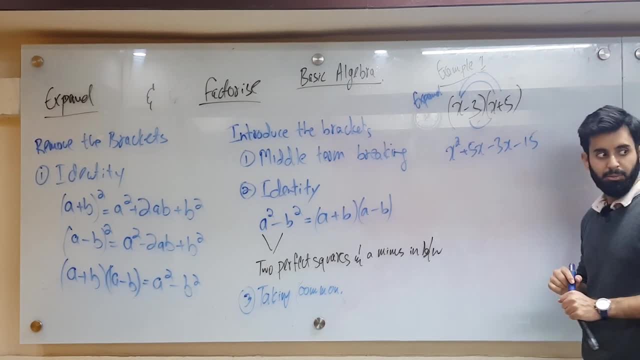 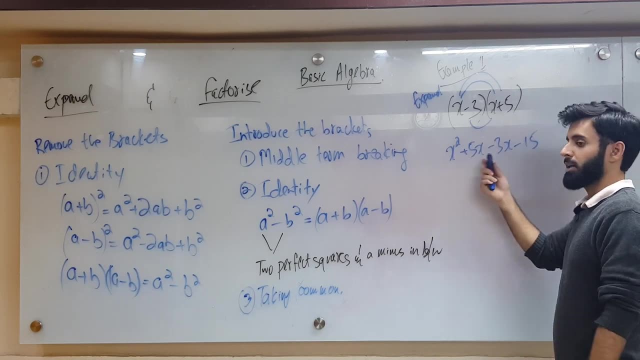 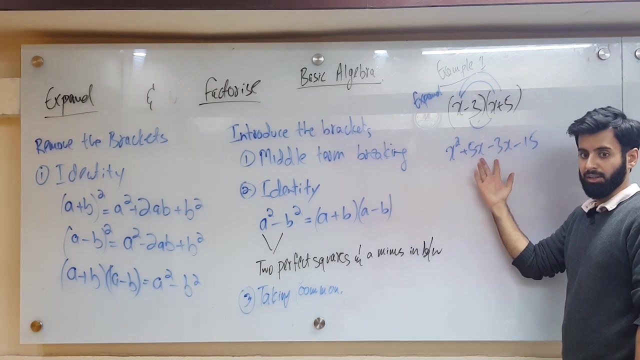 Okay, next you will write expand and simplify. So what does simplify mean? Simplify means that this can be further simplified. Why? Because you have two similar terms that can be added or subtracted. What are those terms? 5x and 3x. So x squared plus 2x minus 15.. 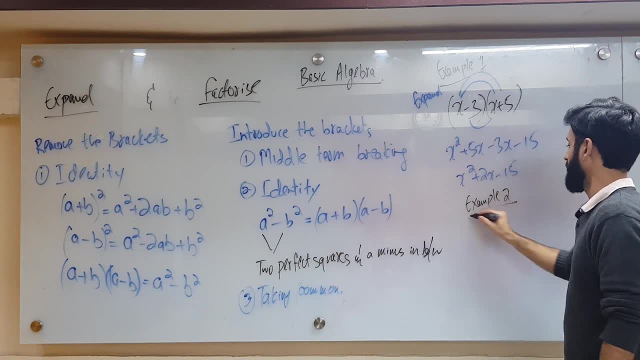 Let's do another example. Alright, what about this? What do you think will be written in this? Expand or simplify, Factorize, No, why will it be factorized? Factorize means to introduce brackets, But there is already a bracket here. 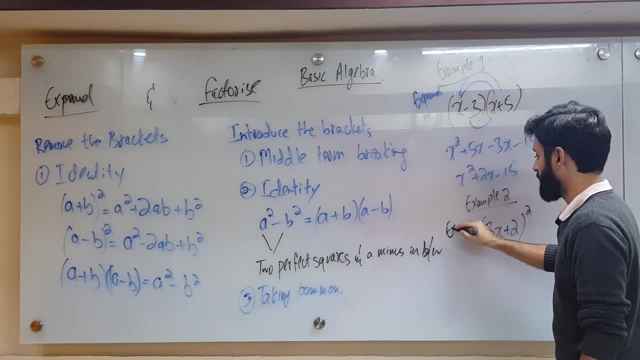 Introduce. So here the question will ask you to do what. The question will ask you to expand. Okay, what identity can I use here? I see two terms, with a plus and a whole square. a plus b, square, a plus b, the whole thing square. 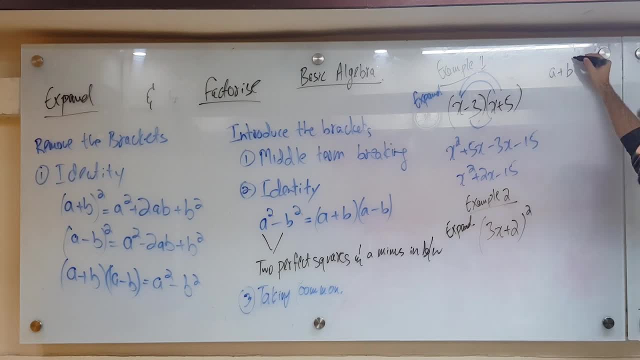 What's the difference between a plus b square and a plus b whole square? If you say a plus b square, you know this is what you are saying: a plus b square. If you say a plus b, the whole square. so this is what you are saying. 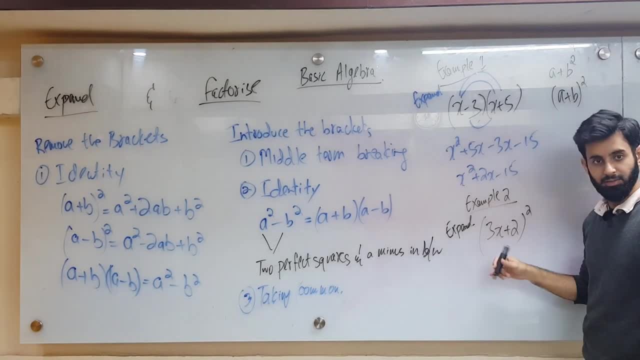 Okay, So what do you see in place of a, 3x, 3x, And what do you see in place of b 2.. So, if I add identity to this, how will I do it? a square plus 2.. 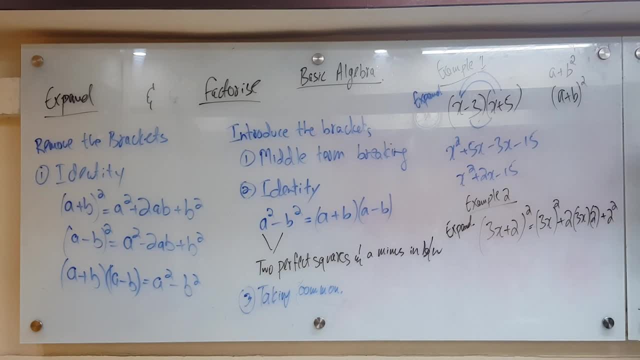 a, b plus b square. Do you understand what I said? This will give us 9x square, plus what's 2 into 3? 6x, 6x. What's 6 into 2? 12x, 12x And what's 2 square? 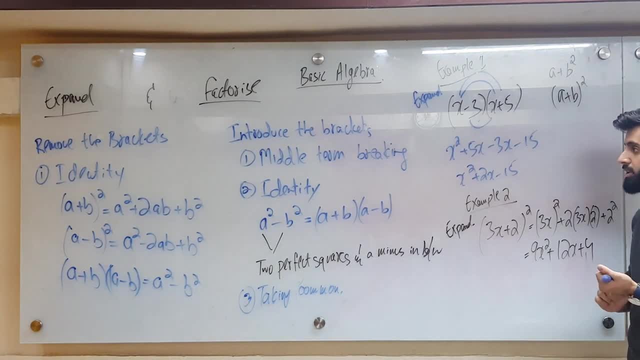 4. Okay, Any questions? Okay, what about this x plus 5 times x minus 5.. What will we do with this? Will we factorize it or expand it? Expand it Again? can I use an identity here? 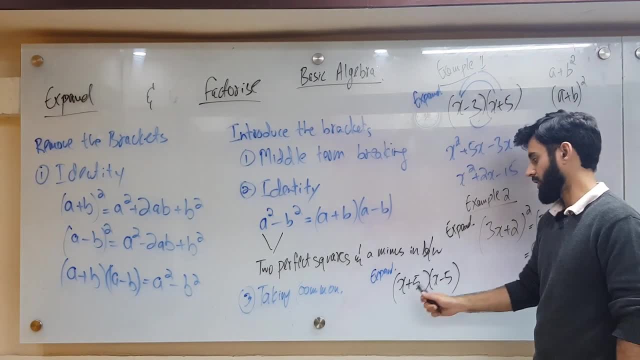 No, No, a square minus b. Yes, What do you see? xb is 5b. The only difference is that in one expression you have a plus sign and in the other you have a negative sign. So we are going to use. 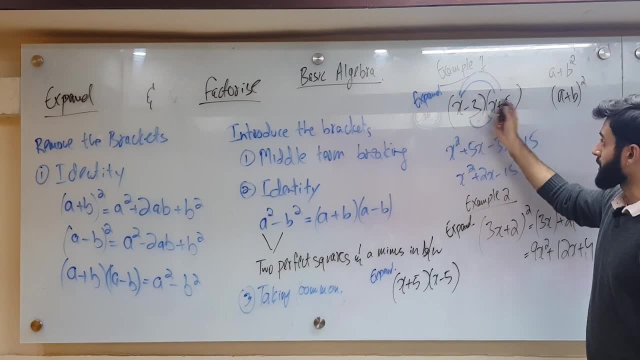 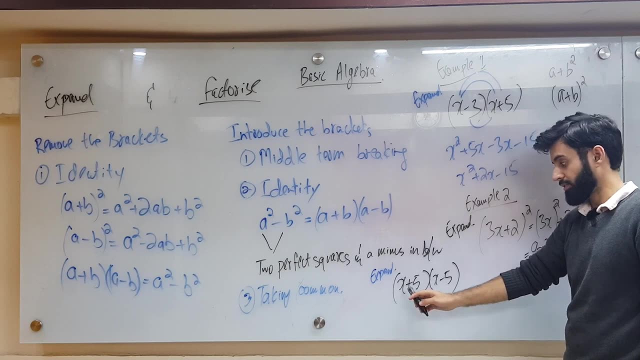 No, It was different. here. The terms were different. here One side was 3 and the other side was 5.. Here both terms are same: xb is 5b, But the only difference is that one bracket has plus and one has minus. 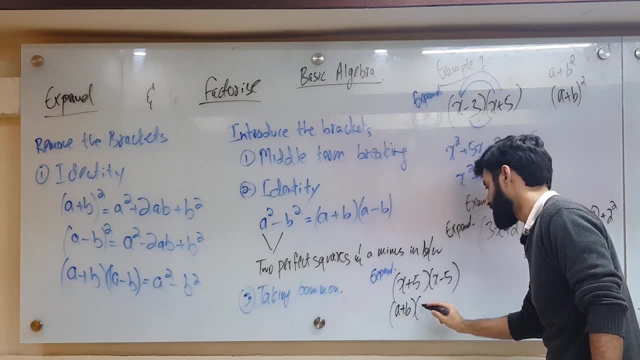 So can I use this identity a plus b, a minus b? Of course I can. If there is a plus sign here and a minus sign there, then it is the same. Listen, when do we use a plus b and a minus b?